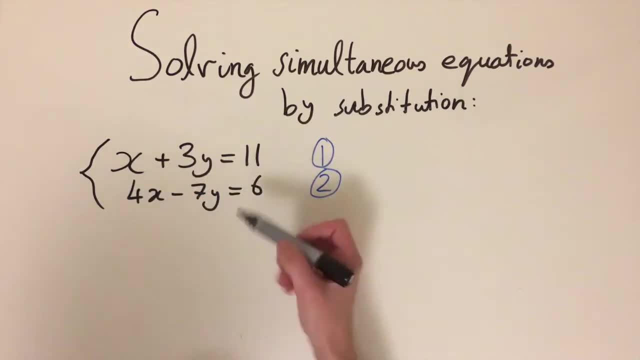 last video. if, for example, we already have a variable isolated on its own- And in this case we do- we have an x with only one coefficient. So our first step is going to be rearranging this equation to find x. So if we do this, we get x equals 11 minus 3y. So let me just 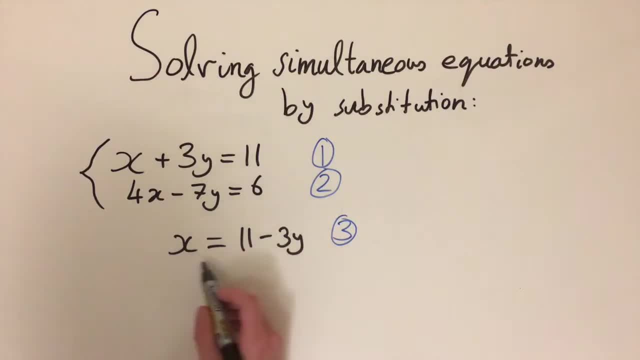 label that equation number 3.. So now we've got x rearranged on its own in terms of y, and the next step is just to substitute it straight into the second equation. So let me just write: substitute 3 into 2.. 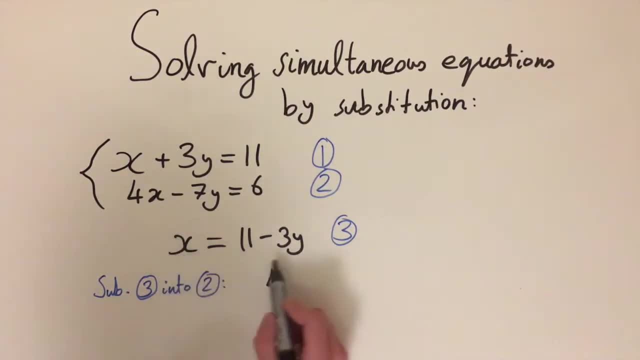 So if we do this, we're going to have 4 times x, and x is now 11 minus 3y, And we still have the minus 7y, and this equals 6 from equation 2.. So now we've got an equation only involving y's, We've eliminated the variable x and 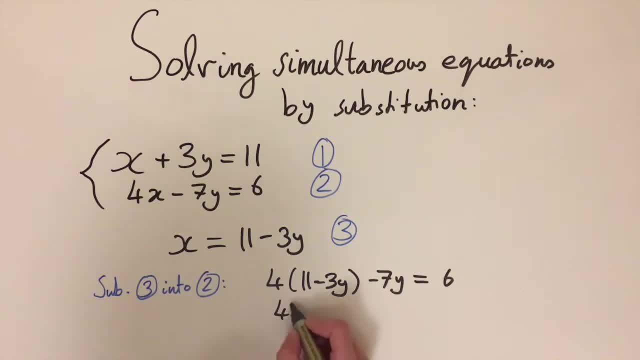 we can solve this very simply. So let's just expand out these brackets. We get 44 minus 12y, Minus 7y, and this equals 6.. So we can collect the terms and simplify This is going to be. 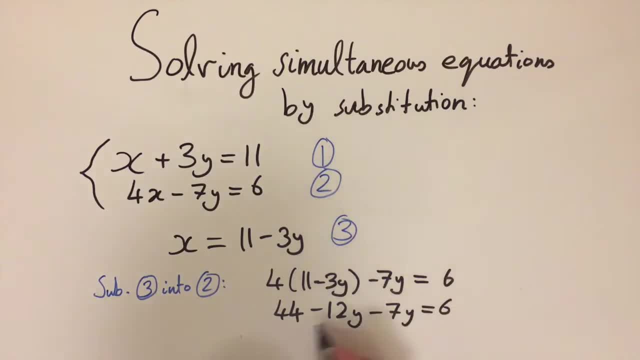 19y minus 19y if we move this onto the other side And then 44 minus 6 is 38. So that's what we get on the left-hand side And the right-hand side we get 19y. And then to find: 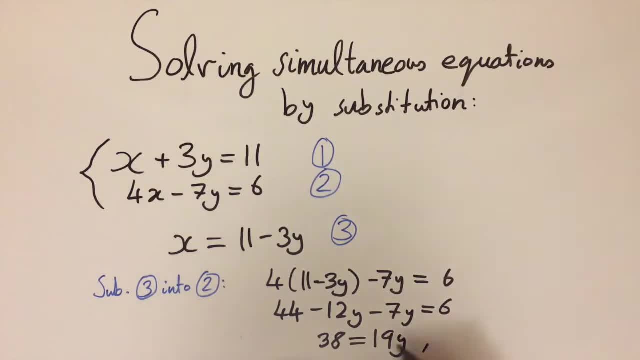 y we just divide by 19.. And 38 is 2 times 19.. So this gives us y is equal to 2.. Okay, so let's go back up here. Let's look at the second equation. Let's go back to the first. 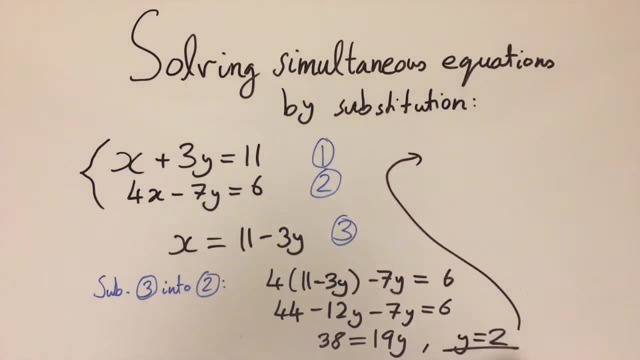 So we've got 14 minus 7y. This is going to be 32.. So we've got 19y minus 19y And then Okay, so let's go back up here for some more space, and now the second task for us to do is to find out what the 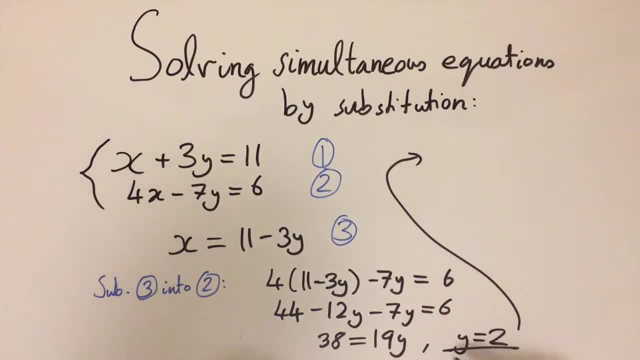 corresponding value of X is. and We're going to do this by substituting y equals 2 into any of these equations. It doesn't matter which one, but we've already got X rearranged on its own, So this is the easiest form. So we're going to substitute y equals 2 into equation 3. 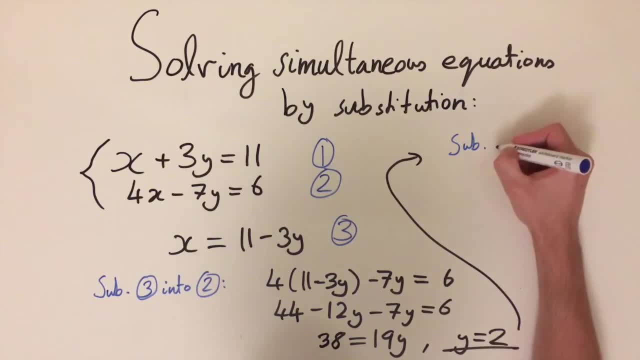 I'll just write up here: Substitute into number 3. So if we do this, we'll have x equals 11 minus 3 times y, and y is just 2, So we have x equals 11 minus. Wait, why did I write 6?? 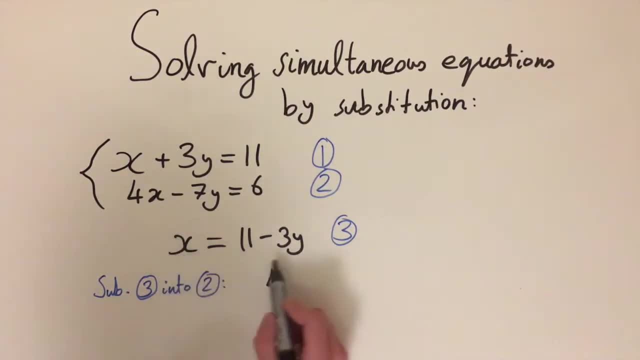 So if we do this, we're going to have 4 times x, and x is now 11 minus 3y, And we still have the minus 7y, and this equals 6 from equation 2.. So now we've got an equation only involving y's, We've eliminated the variable x and 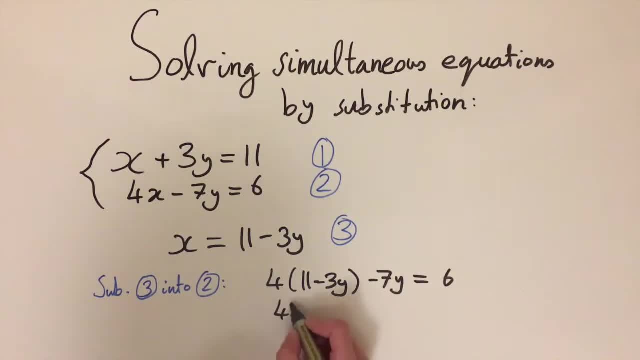 we can solve this very simply. So let's just expand out these brackets. We get 44 minus 12y, 14 minus 7y And this equals 6.. So we can collect the terms and simplify. This is going to be 19y minus 19y if we move. 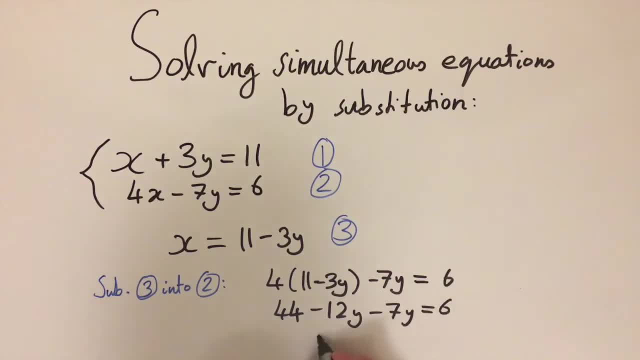 this onto the other side And then 44 minus 6 is 38. So that's what we get on the left hand side And the right hand side we get 19y. And then to find y we just divide by 19. And 38 is 2 times 19.. So this gives us y is equal. 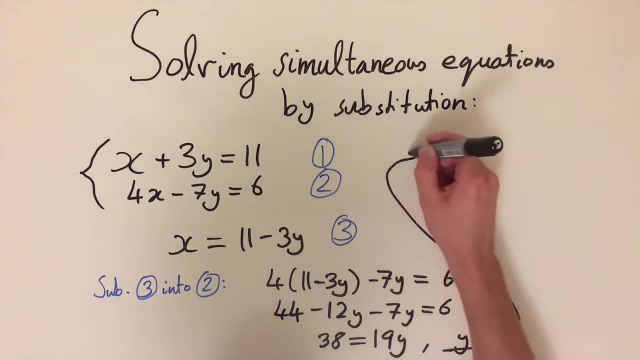 to 2.. Okay, so let's go back up here for some more space, and now the second task for us to do is to find out what the corresponding value of x is, and we're going to do this by substituting y equals 2 into any of these equations. it doesn't matter which one, but we've already. 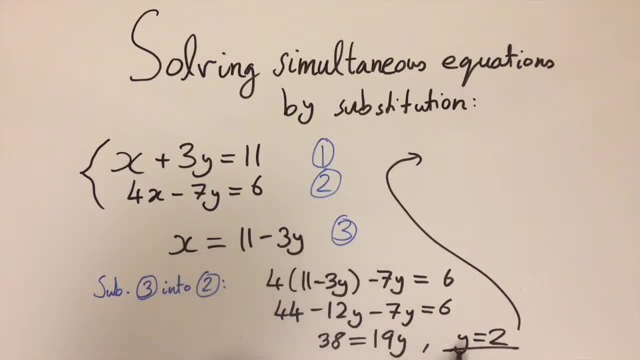 got x rearranged on its own, so this is the easiest form. so we're going to substitute y equals 2 into equation 3.. I'll just write up here: substitute into number 3.. So if we do this, we'll have x equals 11 minus 3 times y, and y is just 2, so we have x equals. 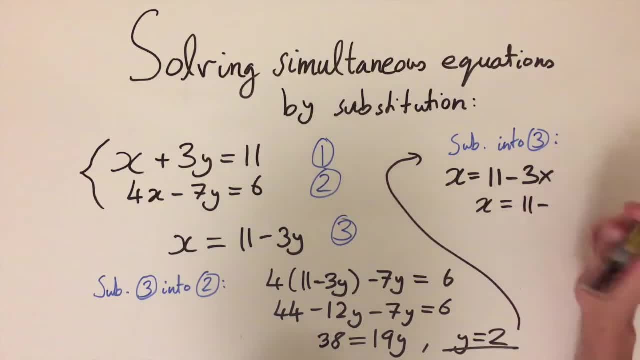 11 minus. wait, why did I write it 6?? 3 times 2, 3 times 2 is 6, so 11 minus 6 and we get y equals 5.. So together, x equals 5 and y equals 2 forms the complete solution of this pair. 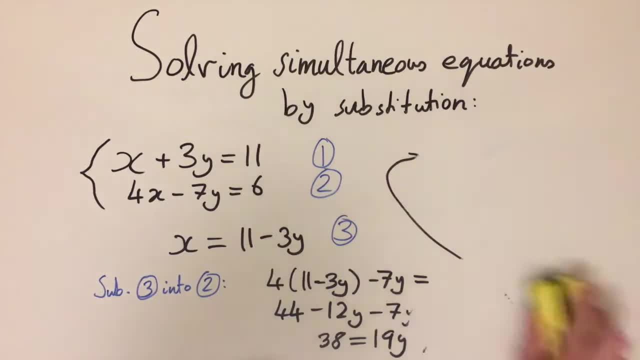 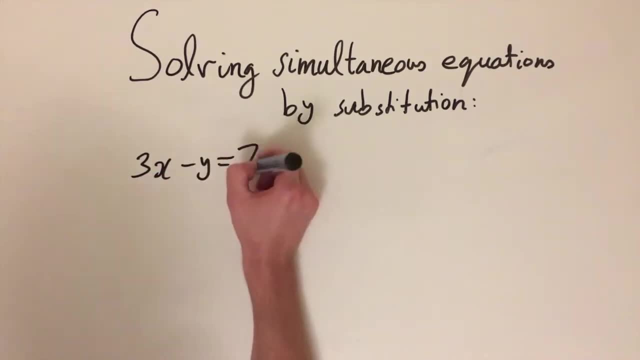 of simultaneous equations. Okay, so let's do one more example. we're going to do: 3x minus y equals to 7. that's the first equation, and for the second one we have: 10x plus 3y equals minus 2.. So these 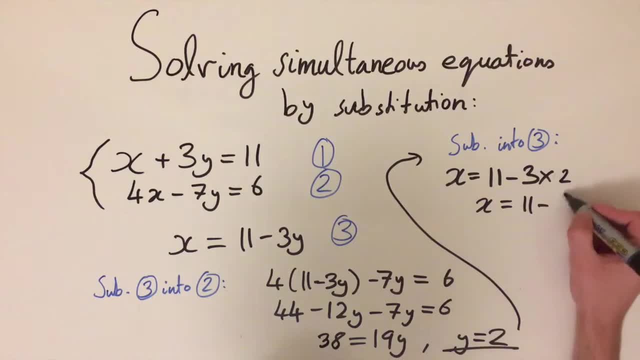 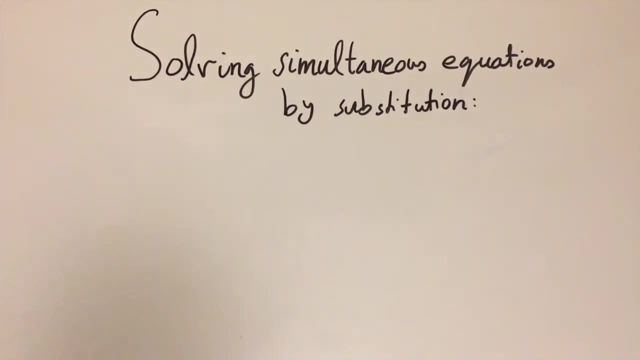 3 times 2, 3 times 2 is 6, so 11 minus 6, and we get y equals 5. So together, x equals 5 and y equals 2 forms the complete solution of this pair of simultaneous equations. Okay, so let's do one more example. We're going to do: 3x minus y equals to 7. 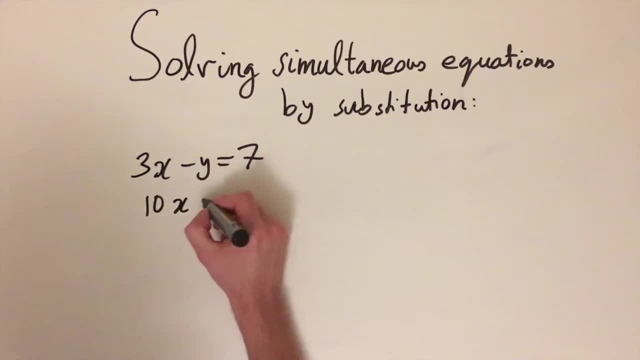 That's the first equation, and for the second one we have 10x plus 3y equals minus 2. so these are two linear equations and we're going to Solve them by substitution. So let me just write this as equation 1 and this as equation 2. 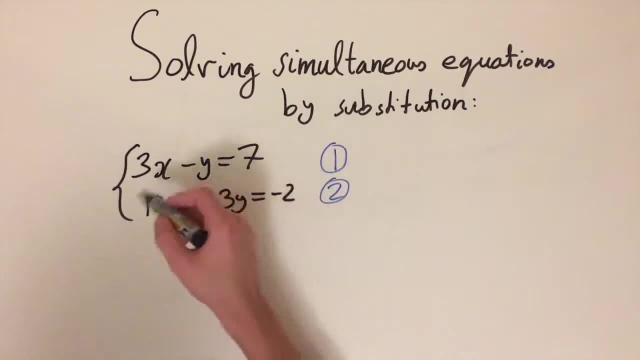 So, just like before, we want to isolate one of these variables, so x or y, as A function of the other one. So here we can see in equation 1 that we only have Coefficient of 1 in front of y. so this is going to be the simplest to rearrange for. 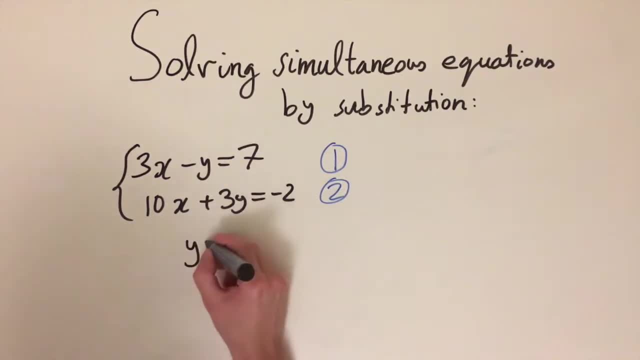 So we can move over the y on to that side, And if we do that we'll get y equals 3x minus 7, and this is just by rearranging equation 1, So it's still equivalent to it. Let's label this as equation number 3. 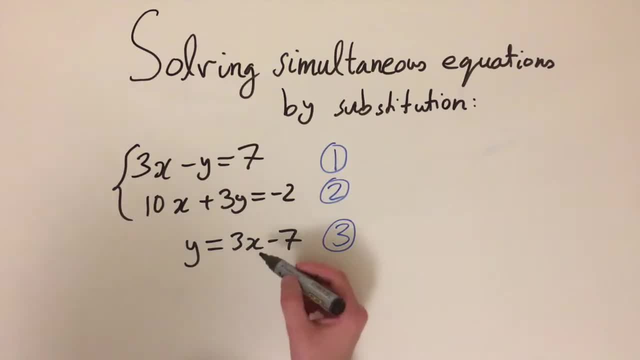 So now we're going to substitute y equals 3x minus 7 into Equation 2, and this is just going to get rid of the variable y. So if we do this, we get x 10x plus 3y, and y is 3x minus 7, and 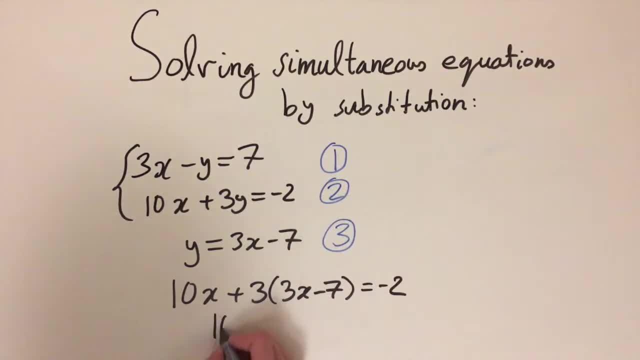 This equals minus 2, so we can expand out the brackets. Get 10x plus 9x minus 3 times minus 7 is minus 21 and this equals minus 2. So if there's any space left over, I'm just going to collect the terms and we'll have. 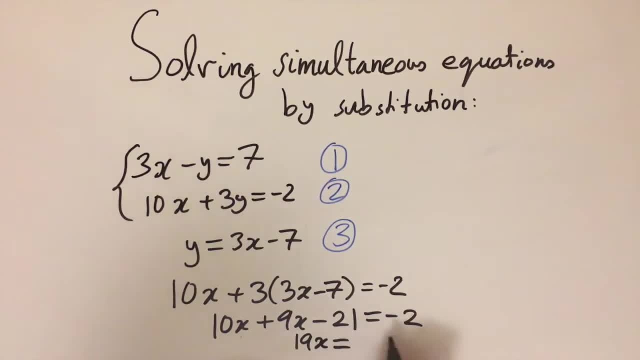 19x equals. and then we move the 21 on to that side and we also get 19. So obviously, just divided by 19, we get x equals 2, 1. And now let's go back up here, And the second stage is just to substitute this value of x back into any of these equations, and let's do it into equation number 3. 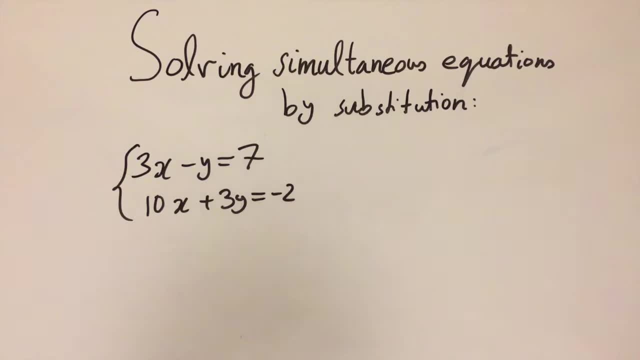 are our two linear equations and we're going to solve them by substitution. So let me just write this as equation one and this as equation two. So, just like before, we want to isolate one of these variables, so x or y, as a function of the other one. So here we can see in equation one: 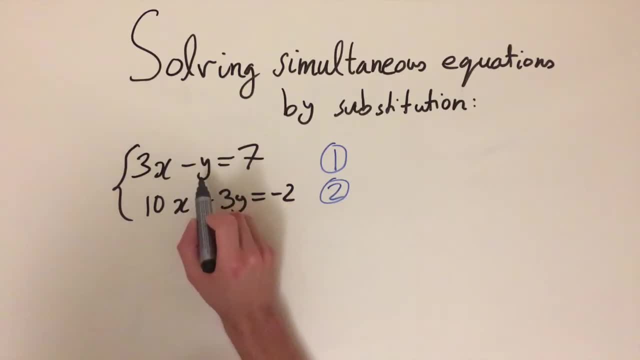 that we only have a coefficient of one in front of y. so this is going to be the simplest to rearrange for. So we can move over the y onto that side, and if we do that we'll get y equals 5. 3x minus 7, and this is just by rearranging equation one, so it's still equivalent to it. 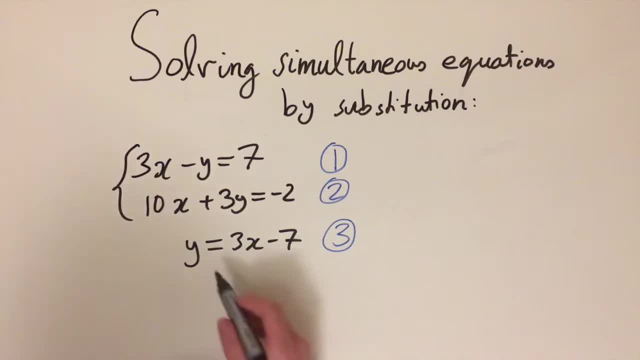 Let's label this as equation number three. So now we're going to substitute y equals 3x minus 7- into equation two, and this is just going to get rid of the variable y. So if we do this, we get x 10x plus 3y, and y is 3x minus 7, and this equals minus 2.. 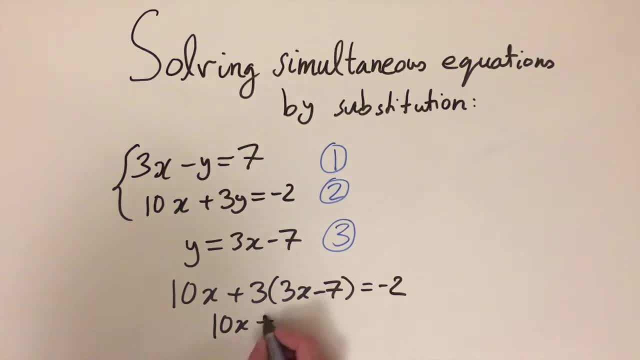 So we can expand out the brackets. we get 10x plus 9x, minus 3 times minus 7 is minus 21 and this equals minus 2.. So if there's any space left over, I'm just going to collect the terms and we'll have. 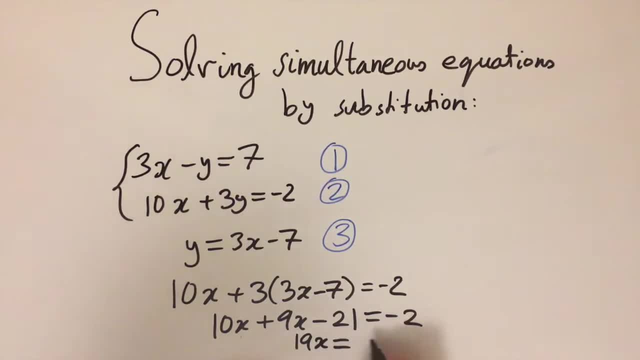 19x equals, and then we move the 21 onto that side and we also get 19. So obviously, just divided by 19, we get x equals to 1.. And now let's go back up here, and the second stage is just to substitute. 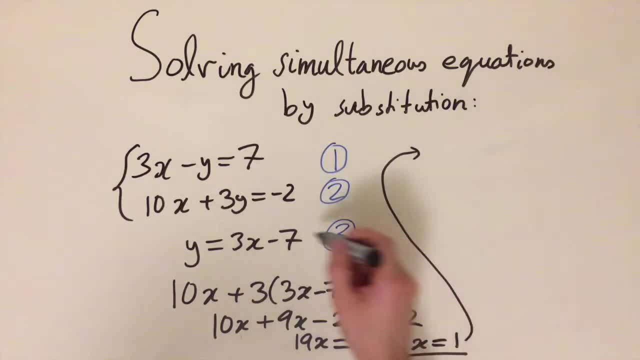 this value of x Back into any of these equations, and let's do it into equation number three. This is the simplest form that we've expressed y in, So we get y equals 3x, x is just 1.. So 3 times 1 minus 7, and 3 times 1 is 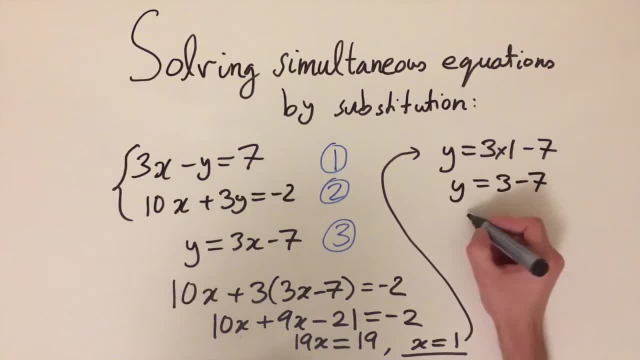 just 3.. So y equals 3 minus 7, and that is also known as minus 4.. So x equals 1 and y equals minus 4 is the solution of this pair of linear equations, And if you wanted to, you could go back into one of these equations and just check that these numbers do add up, and they're. 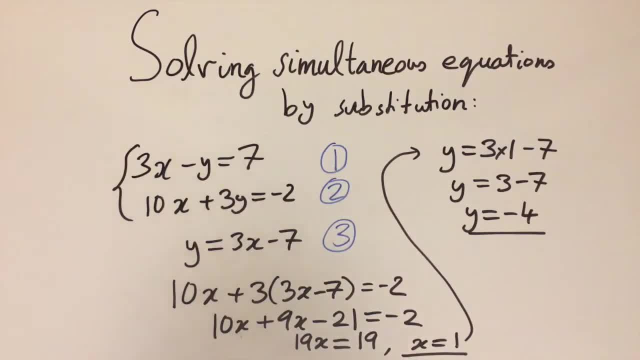 equal, But this is the solution to this set of linear equations.